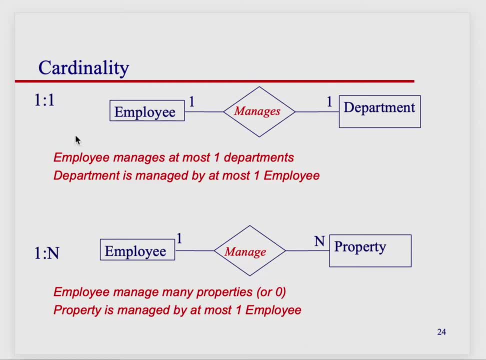 Here in the top example, we have a one-to-one. An employee manages at most one department. So right now you have employee. it's one-to-one. Employee manages a department and a department is managed by one employee And this one is referring to at most. So it's one-to-one. 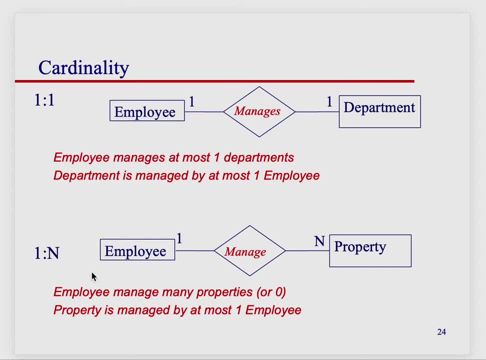 employee manages department. department is managed by an employee, But let's look at a one-to-many example. If we look at a one-to-many example, we have an employee, can manage multiple properties And you also have a property. in this case, of course, a property is only managed by. 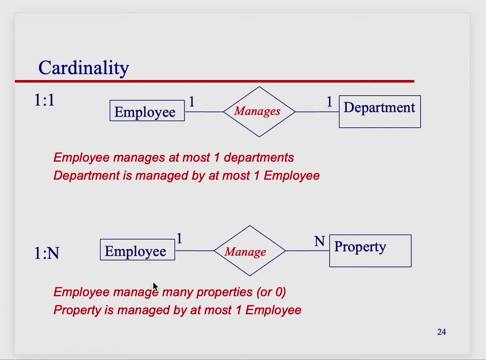 at most one employee. So this is an example of a one-to-many, where a property is managed by by at most one employee. An employee manages multiple properties, so it's one-to-many. If we go to our other two cases now, we have many-to-one. 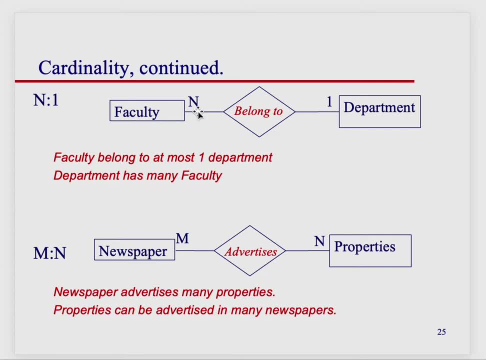 Instead of one-to-many, many-to-one. So faculty belong to one department and a department belongs to. well, a faculty belongs to one department and a department has many faculty. So if you're in this scenario, a faculty member can only belong to one department, at most one department. 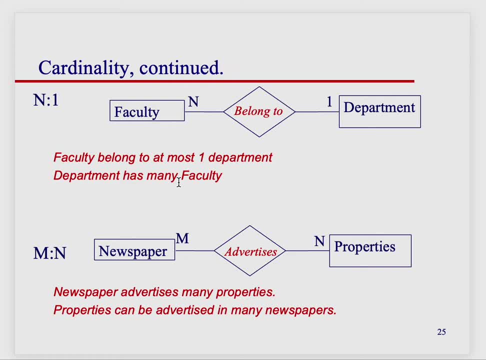 and a department has a lot of faculty. In our last case of many-to-many, we have a newspaper advertises many properties and a property can be advertised in many newspapers. So you see, as I'm reading this, I'm doing like the singular: A newspaper advertises many properties. And then when 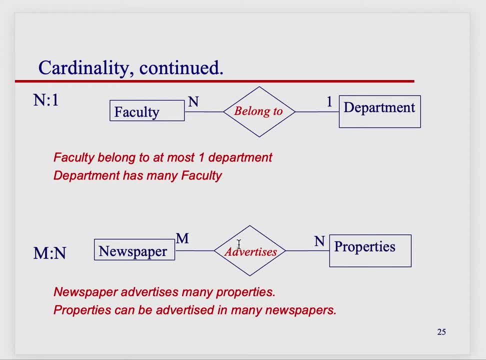 I read it in the reverse. I'm saying: a property is advertised by many newspapers. It could be zero, it could be many, but you can do up to many newspapers if you have an ad that you'd like to place. So this is the example between many-to-many and the example 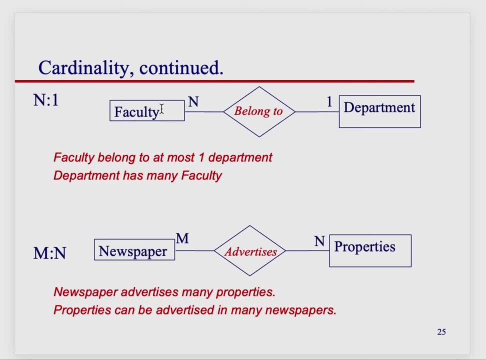 between many-to-many and the example between many-to-one And when we went back to our previous slide, we had the one-to-one and the one-to-many.